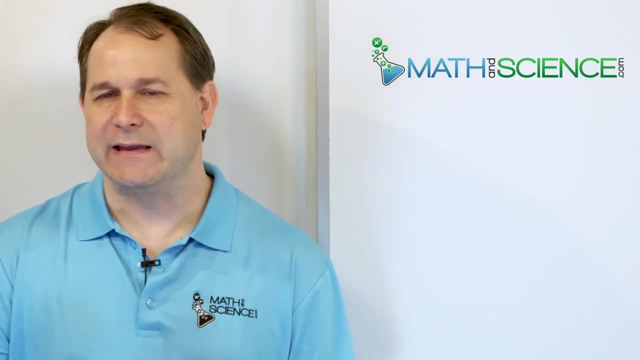 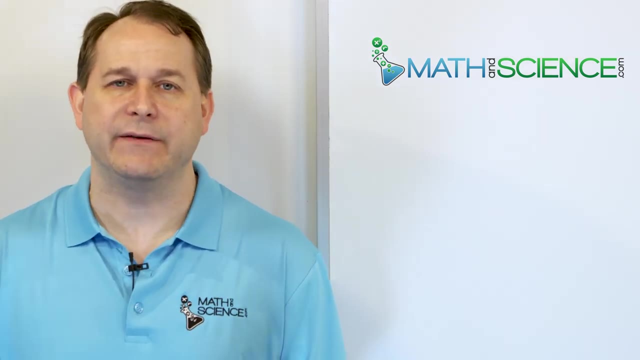 going. This lesson we'll talk about the vertex and the axis of symmetry. In the next few lessons, we'll start working on how to shift these parabolas around the xy-plane, In other words, how to write down the equation of a parabola and, instead of it being centered, 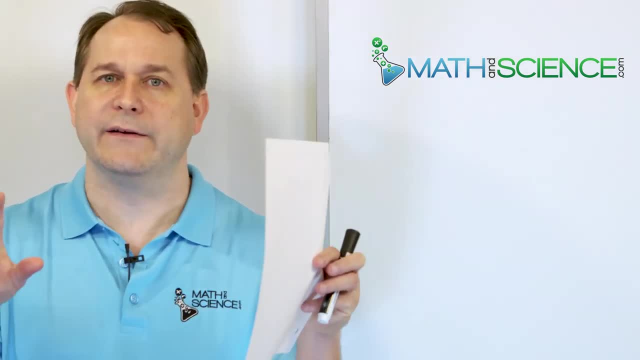 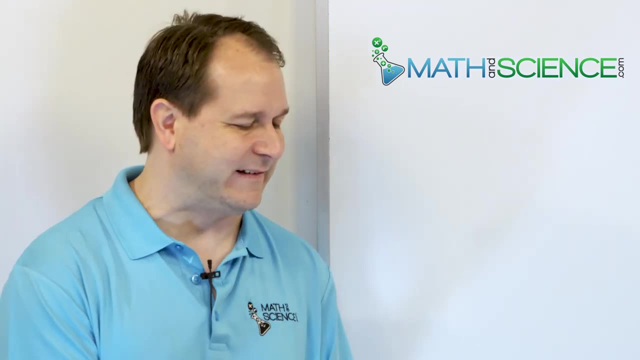 in the center of the xy-plane, how it can be moved left and moved right, and so on. But before we get to that point, we have to understand some ideas and concepts. In this case, we're going to be talking about the vertex and the axis of symmetry. So what I need you to do, 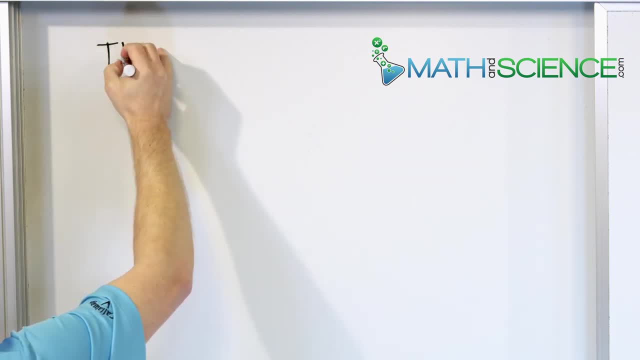 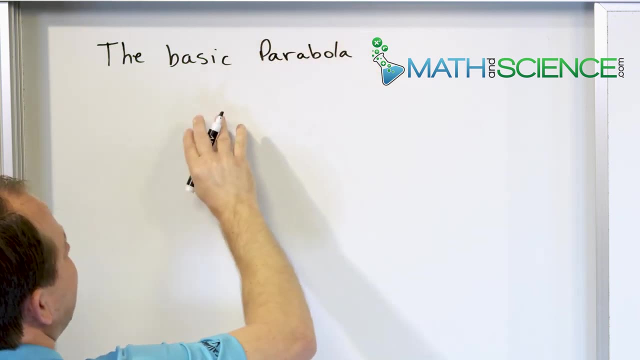 is to understand, really burn it in your mind- the basic parabola. The reason I'm talking about the basic parabola is because in your mind you need to have a general idea, or a very. I say a general idea, but what I mean by that is you need to have a general idea of what. 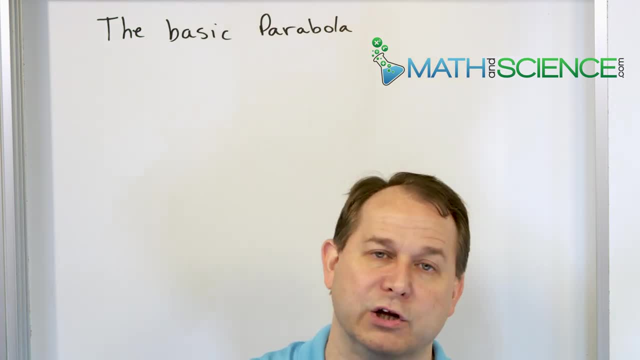 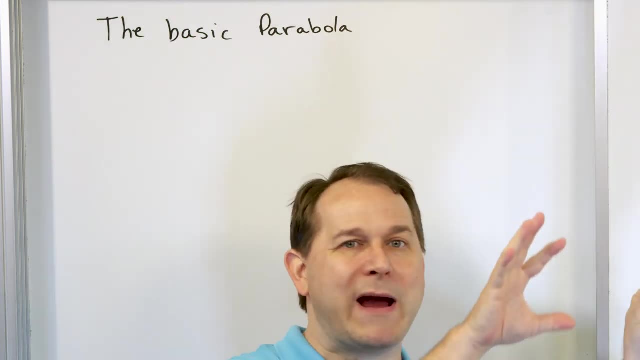 the basic parabola is. You have to burn this image in your mind of what a parabola looks like and where it is centered. I'm going to call that the basic parabola. The reason is because when we start shifting the parabola around, then all we're going to do is take. 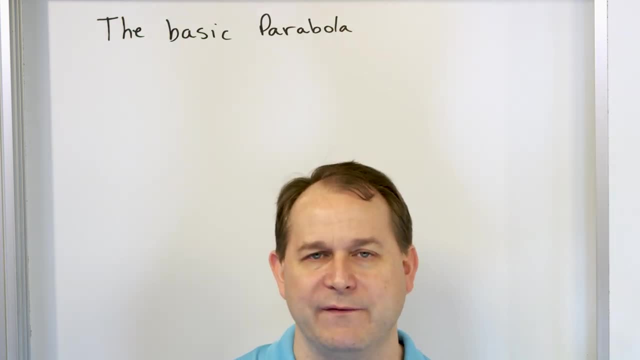 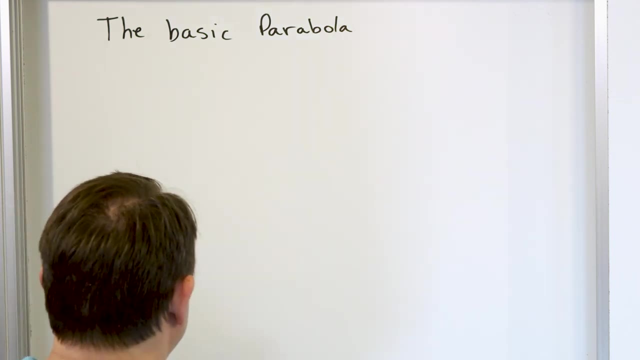 the original equation of the basic parabola and change it very slightly in order to move it around. So we have to have an idea of what the basic one looks like. So you've already encountered this. We've talked about it many times before. The basic parabola is very simple. 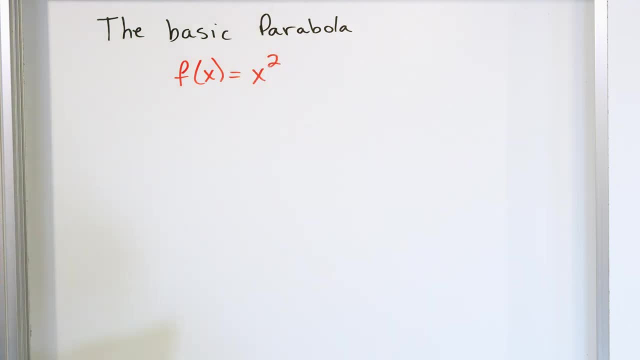 F of x is equal to x squared. This is the most basic parabola that we've ever seen. This is the most basic parabola that you can get And if you don't want to think about functions, you can write it. instead of f of x, You can say that y is equal to x squared. 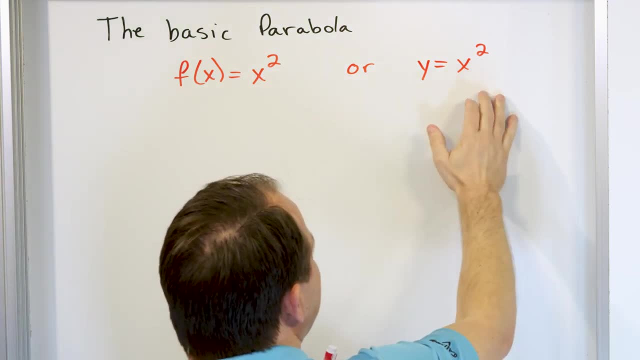 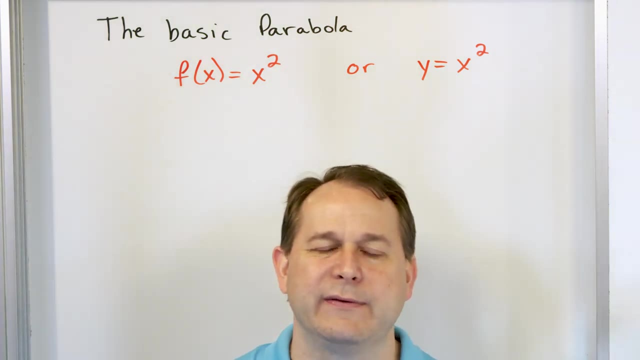 Usually, when you start algebra, you look at it in terms of y is equal to x squared. And then later on, we understand the concept of a function, And so you replace the y with f of x, But functionally, these two things, these two representations, are saying the same. 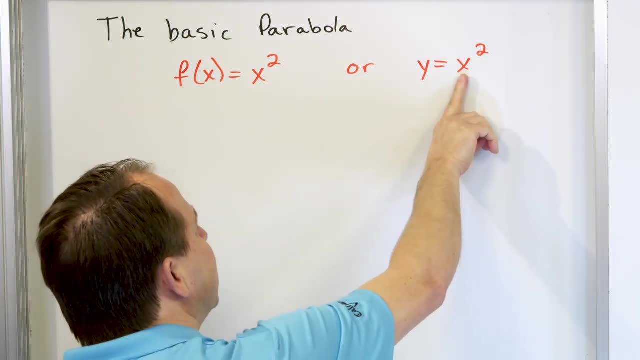 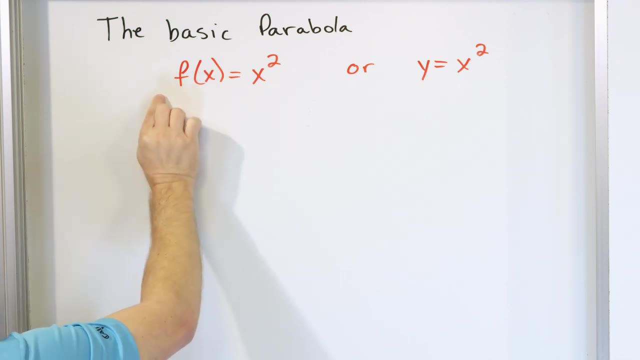 thing. What they're saying is that we stick numbers into this side of the equation and we square them And then the result gets applied to. in this case, it's a variable y. In this case, it's a notation which is a little more clear, saying that this function is a. 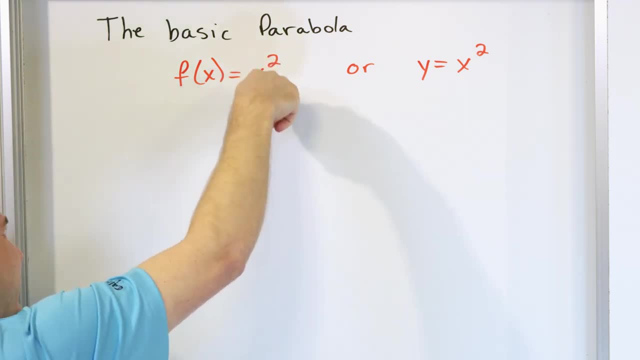 function of x, because x is what we're changing, And then the results kind of get spit out there, And we've talked about the idea of what a function is in the past. So we're not going to do this for every single problem, But for this one, because the basic 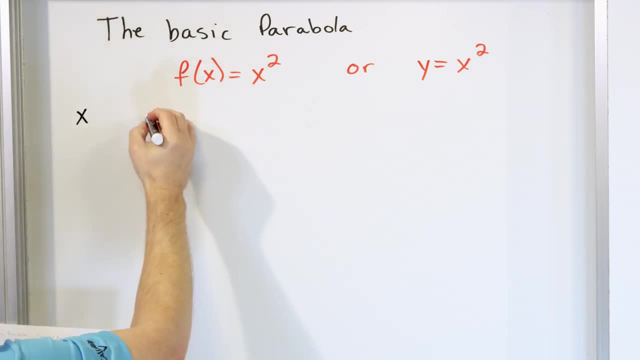 parabola is so important. I want to write down a few points. So we have x as an input And then we have- I'm going to use the y notation- y is equal to x squared, So we'll just make a quick little table. 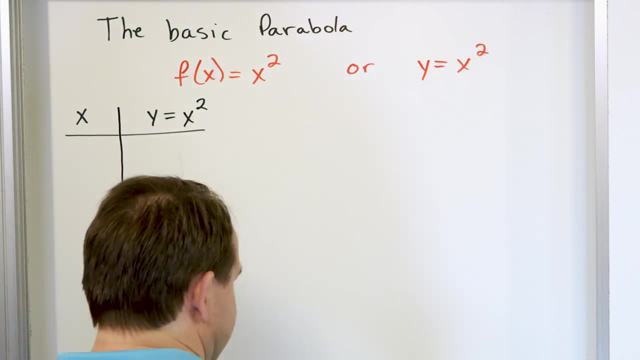 We've done this before, but I just want to do it here, because we're going to graph it as best we can And then we're going to play around with it and kind of like. so in the case of that, we need to have an idea of the basic problem in our mind. So we need to pick. 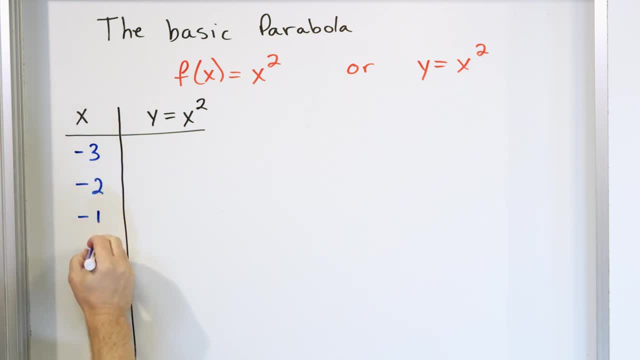 some points. So let's go from negative 3, negative 2, negative 1, 0, 1,, 2, 3.. Of course, you could go all the way to negative 5 or negative 10 or positive 5 or whatever, But 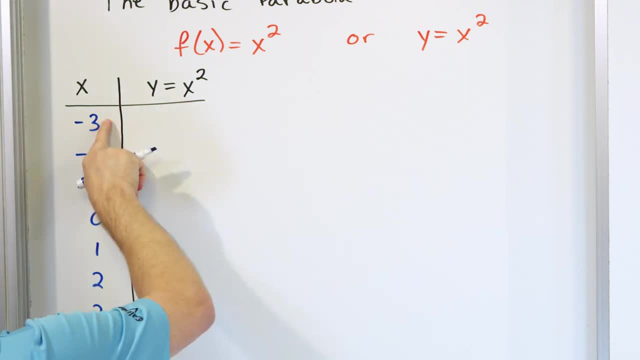 in this case I'm just going to stick to negative 3 to positive 3.. So when we take a negative 3 and we square it, negative 3 times negative 3 just gives us a number. Negative 2, we square it, we get a positive 4. Same thing here: we get a positive 1. Zero. 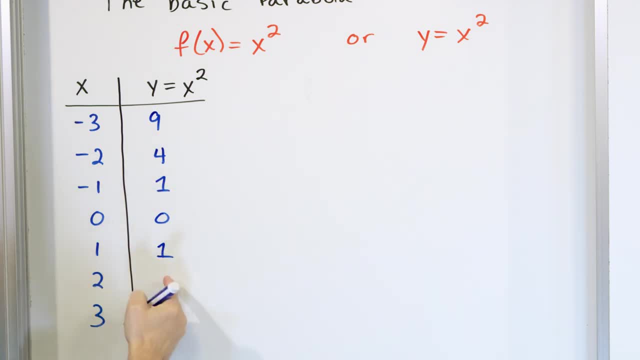 squared is a 0.. One squared is a 1.. Two squared is a 4.. Three squared is a 9.. So right away, before we even graph anything, you can already see some symmetry in the shape of the parabola. 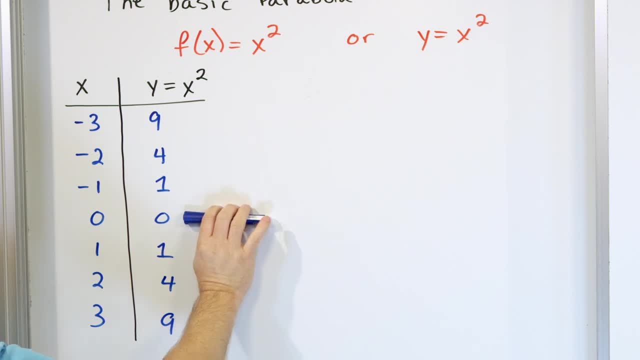 The center of the thing is basically here: If we go to positive values of x like this, then we get larger and larger outputs, which is the y values. But if we go to the negative values of x, We get the exact same outputs as in the other side. The 1 matches with the 1, and so on. 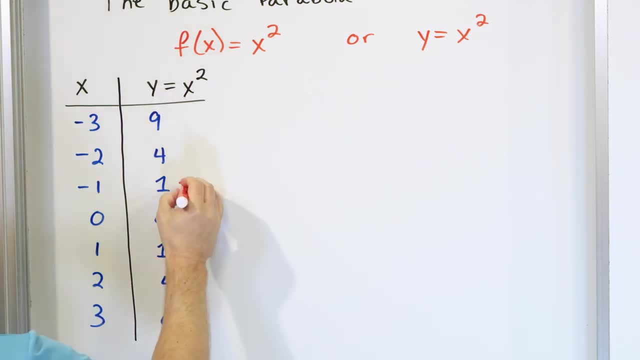 So I can kind of like, just kind of like make it super obvious: This one goes with this one, this one goes with this one, and the 9 goes with this one, And so we say that the graph of the parabola is symmetric, And we'll see it a little more clearly when we draw it. 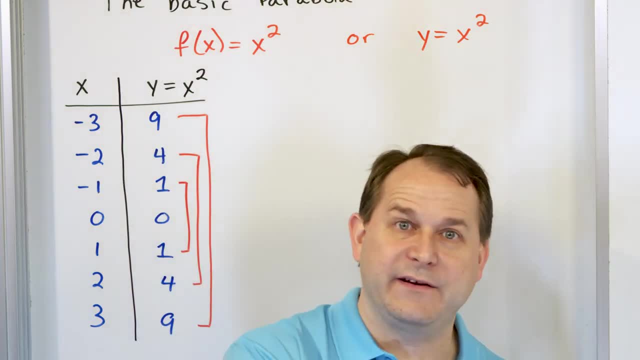 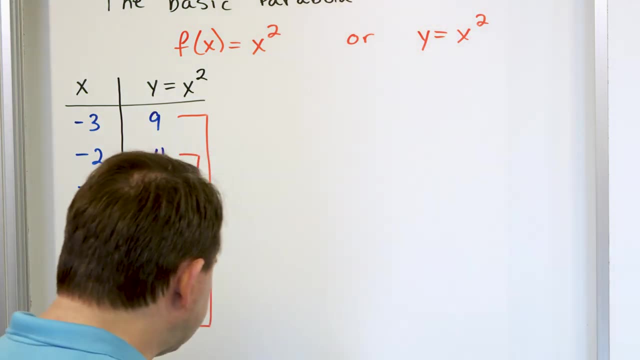 But basically, whether you go to negative x values or positive x values, the outputs of the function give you exactly the same thing. So it's like a mirror image, right? So let's go ahead and draw this graph. It doesn't need to be perfect, I'm not going. 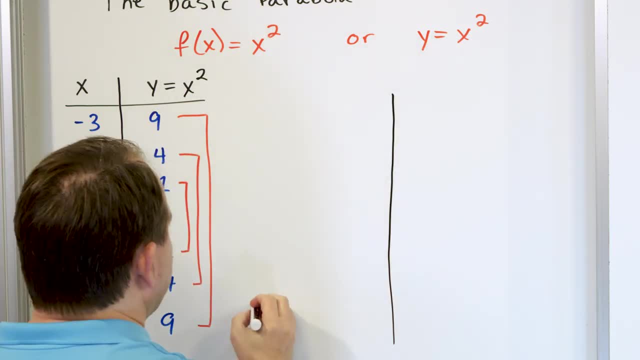 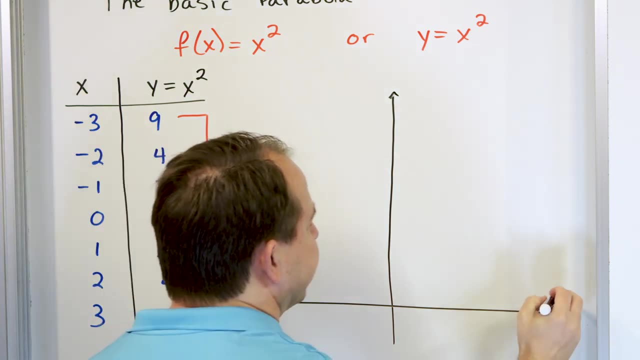 to pull out the crazy graph paper or anything like that. We're just going to, in general, write down what we need to burn the image in our mind of what this parabola is. So here we have x And here we have. I can put f of x, here I'll just put y, since we're doing. 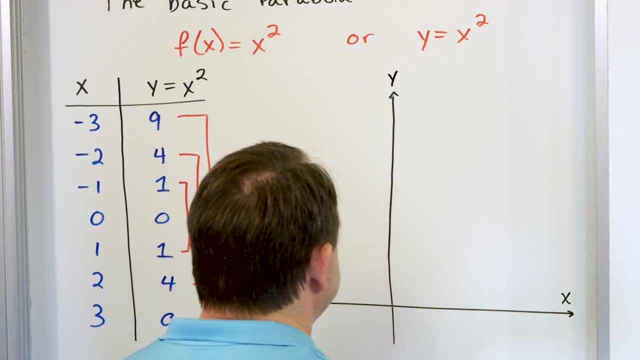 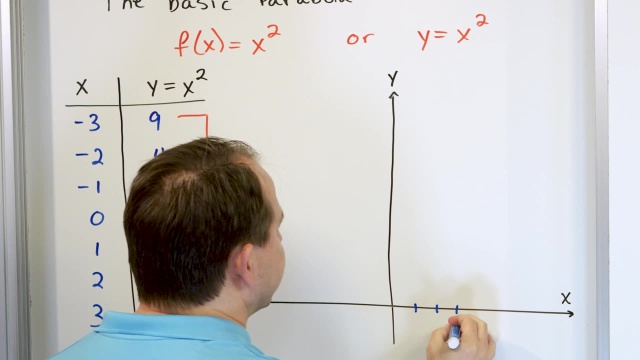 everything in terms of y, And then we need to have some kind of tick marks, right? So again, I went from in my graph here, negative 3 to positive 3.. So let me go 1,, 2,, 3.. So 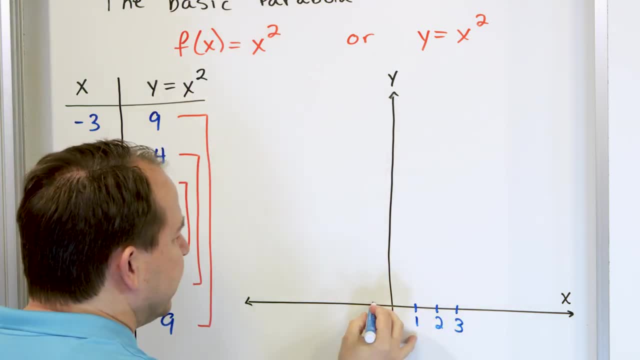 this is 3.. This is 2.. This is 1.. This is 0.. This is negative 1, negative 2, negative 3.. So I'll put negative 3, negative 2,, negative 1, right. 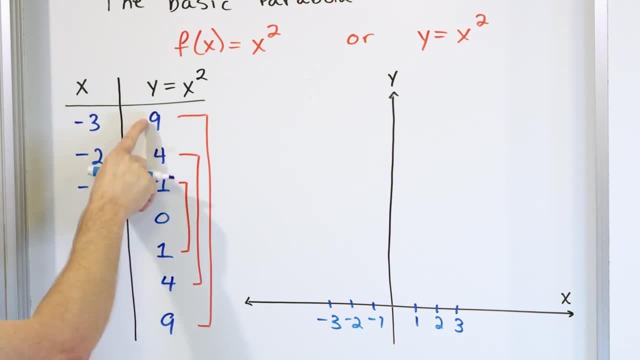 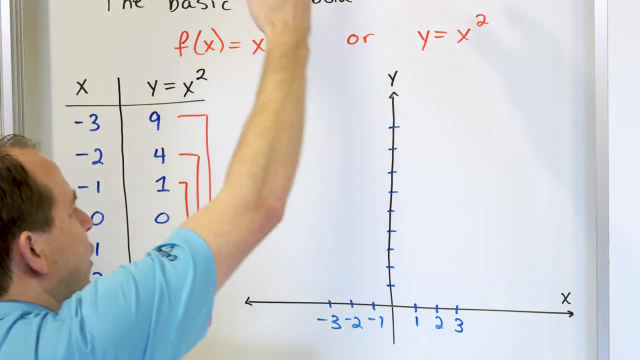 And then, when I graph this guy, I ended up getting a large value of 9.. So I'm going to go ahead and put 9 tick marks: 1,, 2,, 3,, 4,, 5,, 6,, 7,, 8,, 9.. I could go on, of course. 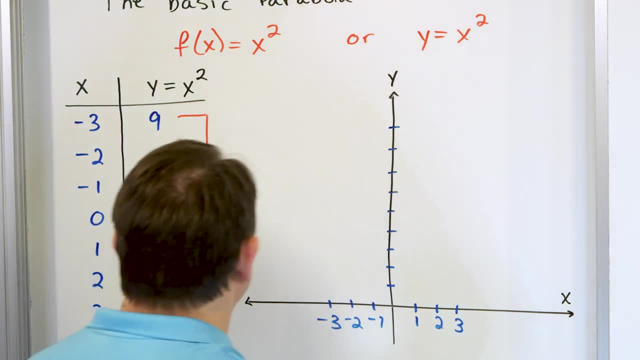 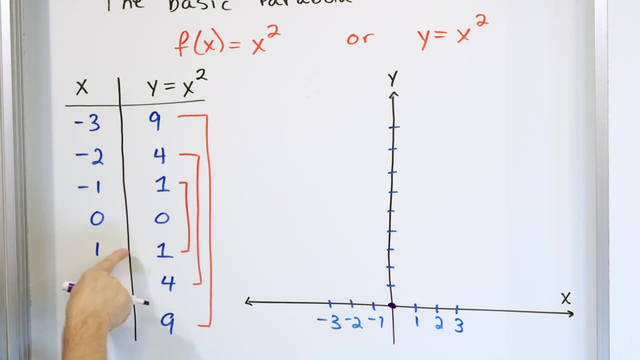 but I don't have any points that are beyond that place. So let's go ahead and plot this thing. We have x comma y, which is 0 comma 0, which means we have a point right here. We have 1 comma 1,, which means we have 1 comma 1 right. 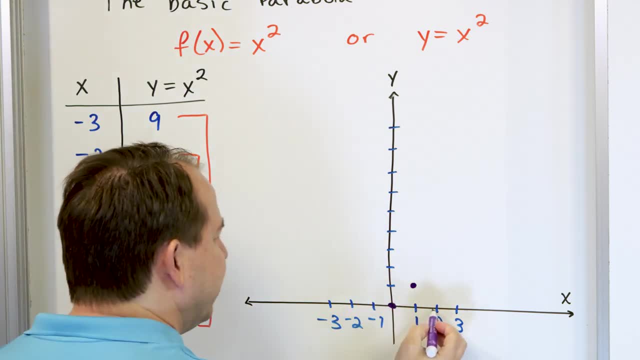 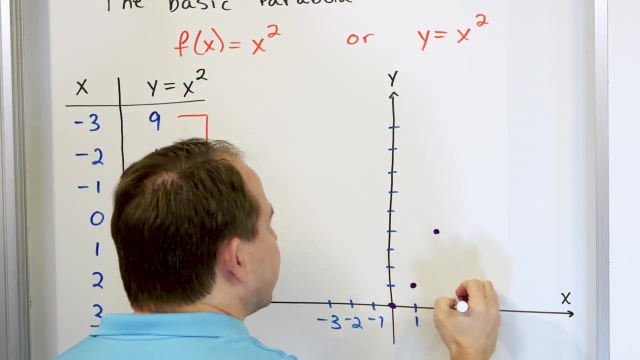 here We have 2 comma 4,, which means we have 2 comma 1,, 2,, 3,, 4.. So that one is actually somewhere right around there. And then we have 3 comma 9,, which means we have 3.. And 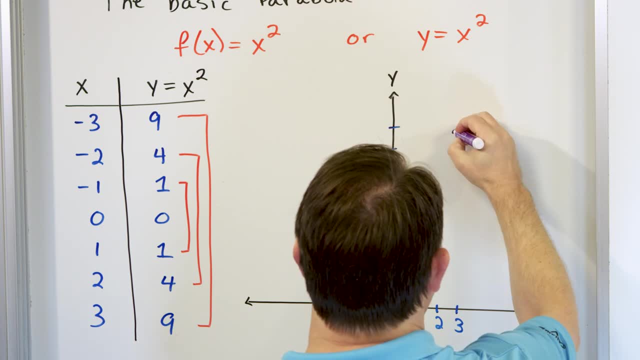 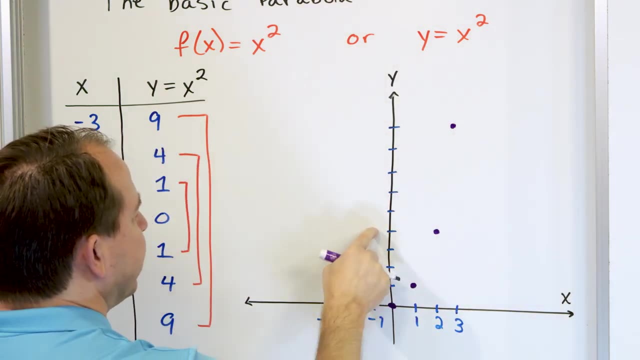 if I've counted correctly, let me stand in front to try to get it to look as good as I can get it. It's not perfect, but let's put it a little bit higher somewhere right around here. So 1,, 2,, 3, 4,, 5,, 6,, 7,, 8, 9 is where that point is. 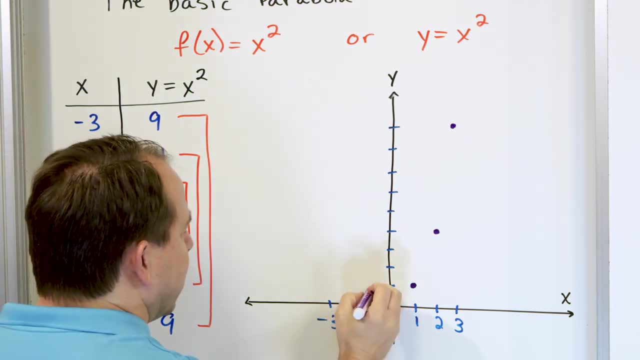 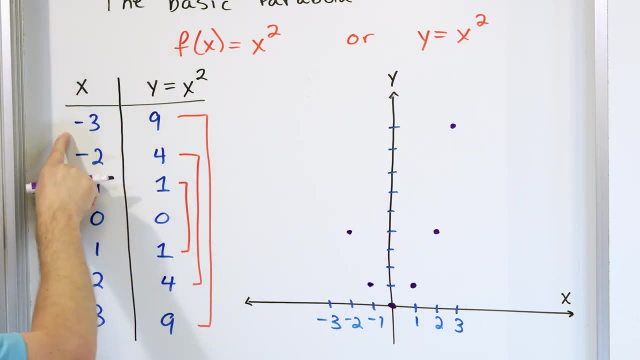 Now let's go the other direction. Negative 1 comma 1 means negative 1 comma 1 is right here. Negative 2 comma 4 means negative 2 comma 4 is right here. And negative 3 comma 9 means let me stand in front so I can try to line it up as good as I can. That's something. 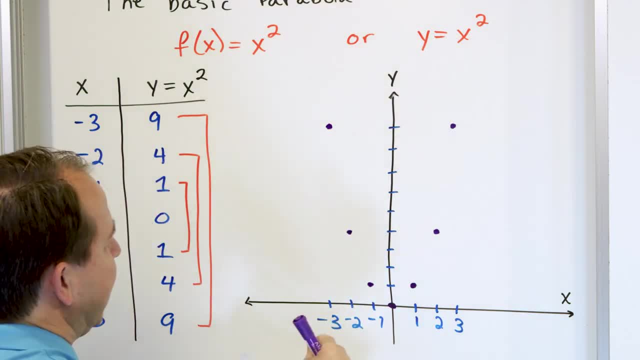 like that. It's not exactly right. So you see, this is not a straight line. If you try to draw a straight line through these two points right here, then you don't hit this one. So you can see it's a curved kind of thing. So I'm going to do my best to sketch it. but 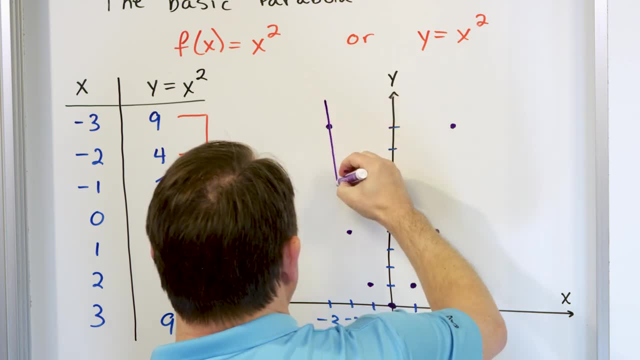 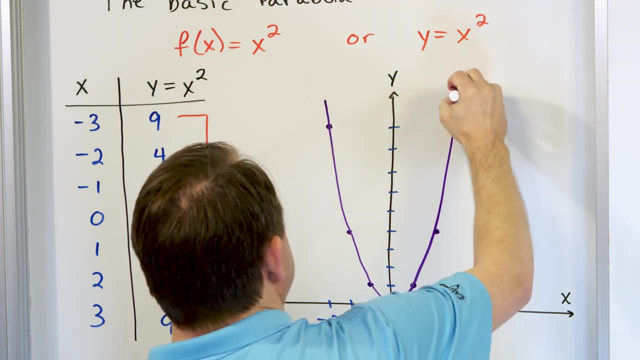 just keep in mind that it's not going to be perfect. So let's go down here, through these two points. We bend over, we go down here, we go up through these points like this. Of course I could go off to the computer, but the point is, when you're on your, when you're 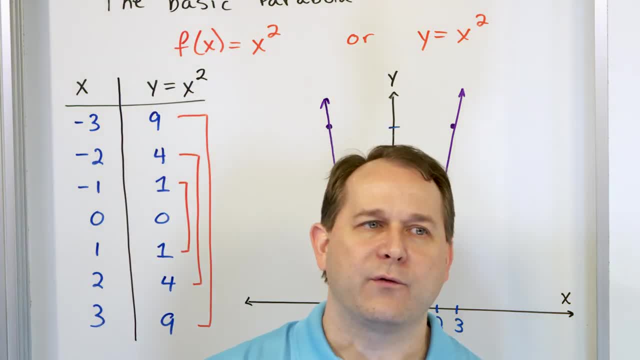 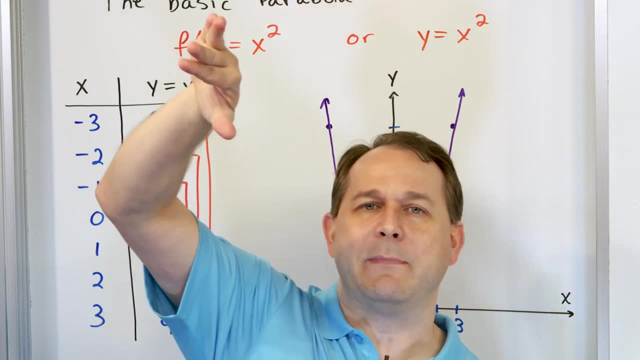 on your paper when you're on your exams. you're not going to have a computer, right? So of course I could show you a computer image, and I have shown you already computer images of what a parabola really looks like. It's a beautiful curve that goes down like a smiley. 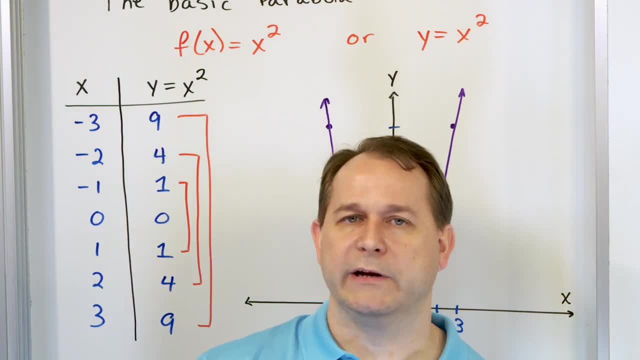 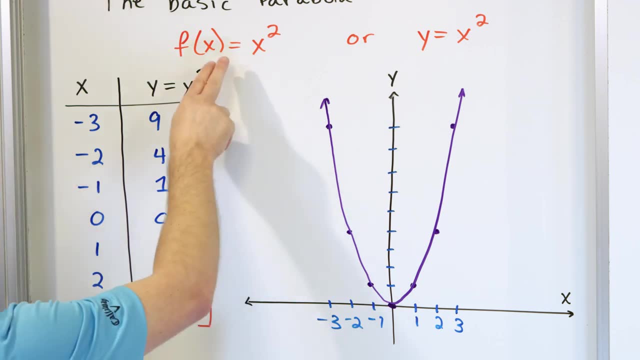 face kind of, And then it goes up for the, for the one that opens upward anyway. But for this I want you to burn this image in your mind. This is the what we call the basic parabola. It just is F of X is equal to X squared, or Y is equal to X squared, And we plot the points. 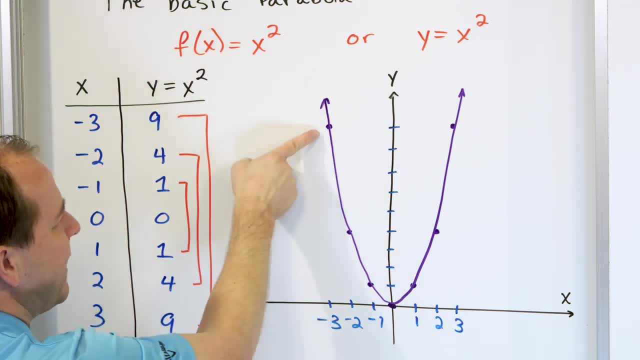 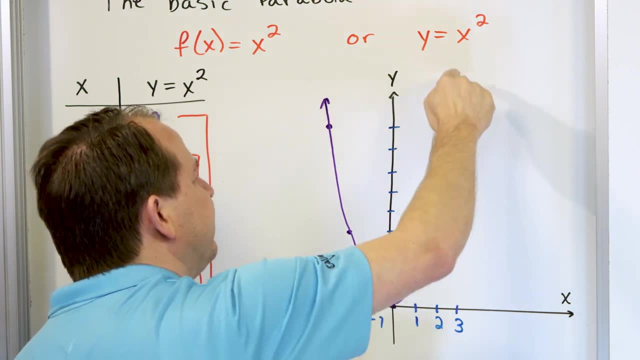 like this to show you the general shape of the thing. But just keep in mind, between all of these points there are infinite points in between all of these points which I could of course fill out in the table there. that would trace out the shape perfectly. And of course I could go on and on forever writing points down. But 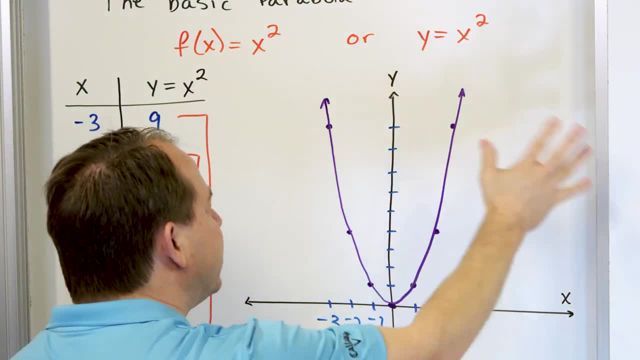 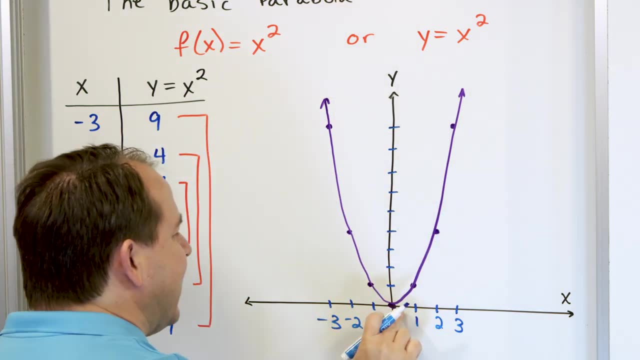 the purpose of this is not to be exact and it's not to put a million points on. The purpose of it is so that you can see the basic shape. What can we learn from this? right, This parabola has a lowest point here. right, And this point here is called, has a special name. It's called 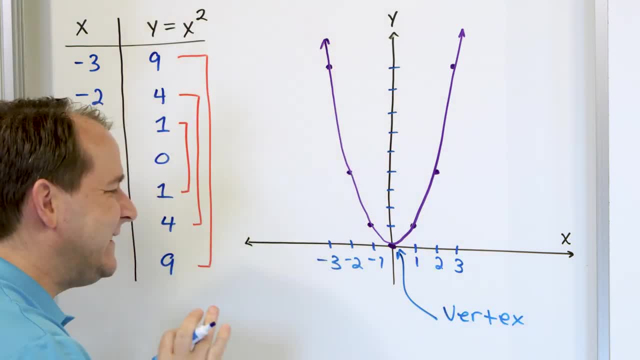 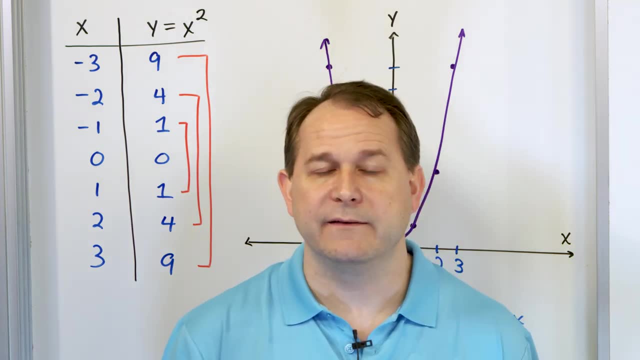 the vertex. So anytime when I say or a book says, or a teacher says the vertex of the parabola is located at blah, blah, blah, All it means is that's the lowest point of the parabola. Okay, 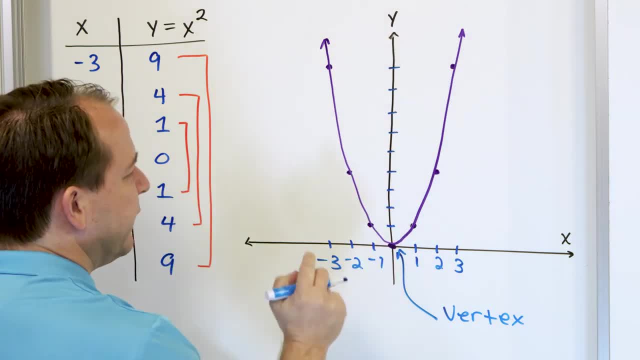 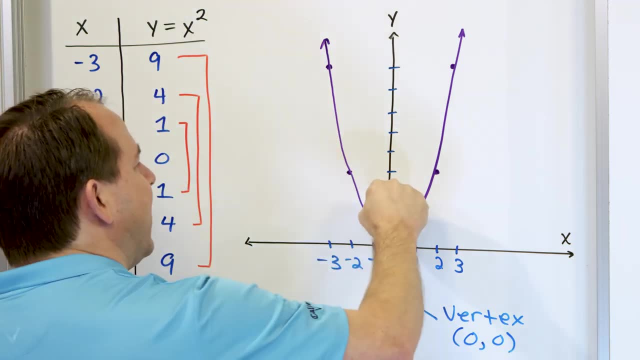 And, of course, I've drawn a parabola that opens up like this. So the lowest point is the vertex, and this vertex is located at zero comma zero. Now, later on, we're going to grab this parabola and we're going to move it all around, So I can have the parabola over here, or I can. 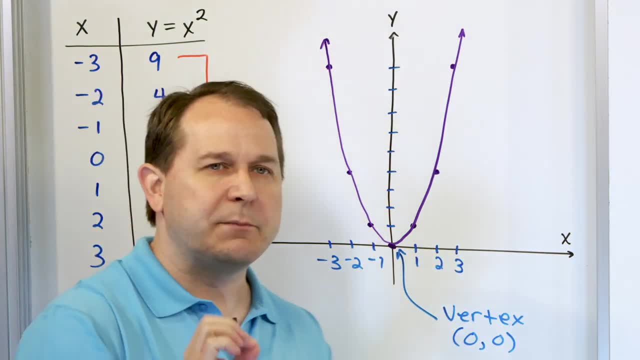 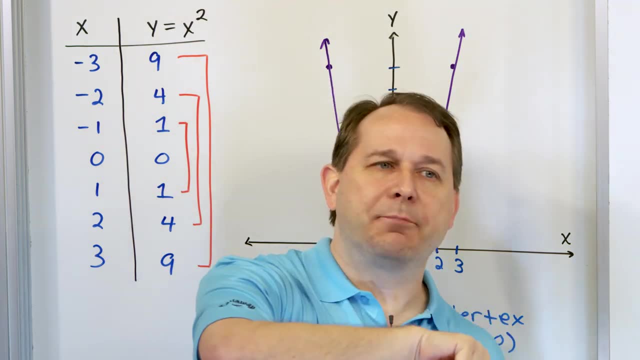 have the problem over here. I can have the problem over here. The vertex of the parabola will just be the point at the lowest part of that parabola. If it opens up like this- we'll see in a minute- the problem can actually go upside down, in which case the vertex will. 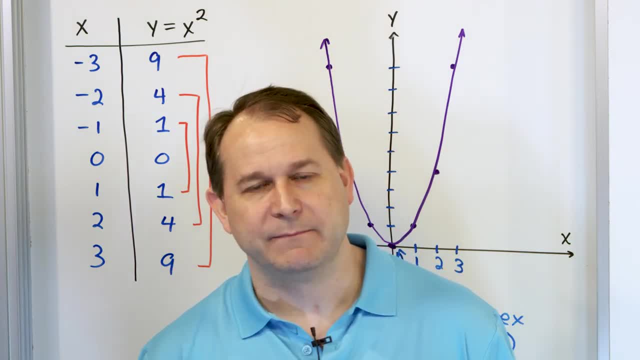 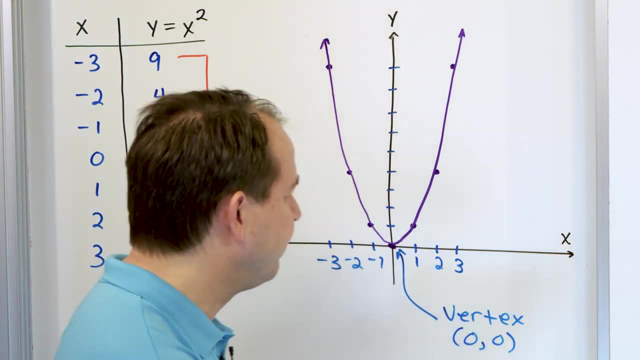 be the tippy top. So we're going to call that the vertex of the parabola or the minimum value of the parabola, like it is here. But either way it's called a vertex and it has a coordinate point, in this case, zero comma zero. 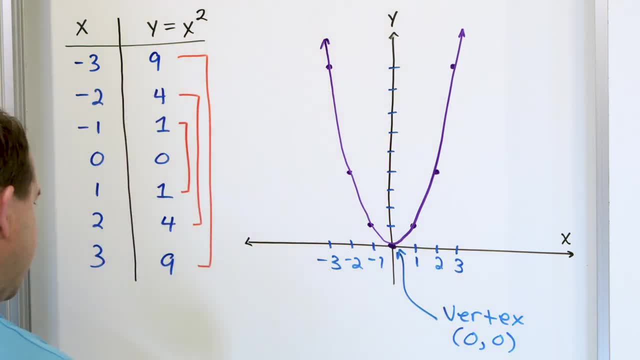 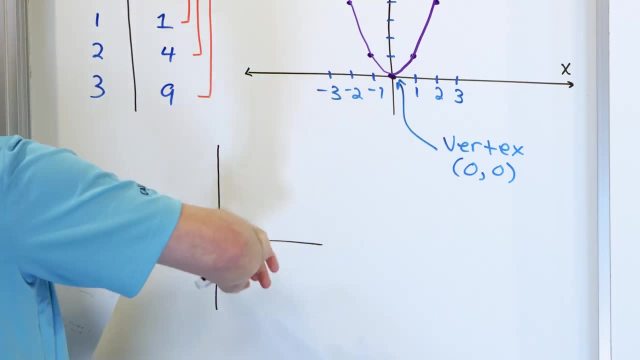 So for the basic parabola, the vertex is located at zero comma zero And, as I've already hinted, we can of course have parabolas drawn all over this plane and they can open up or they can open down. Let's say I had a parabola that went and opened upside down, like this: 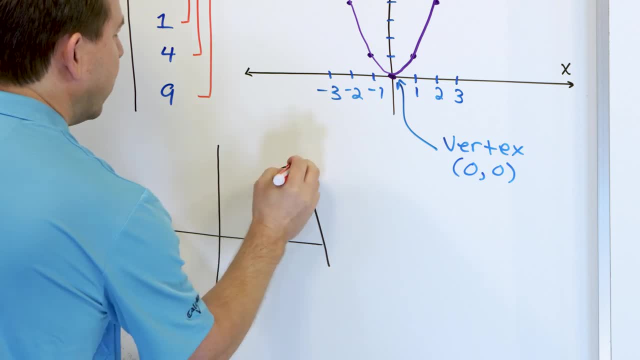 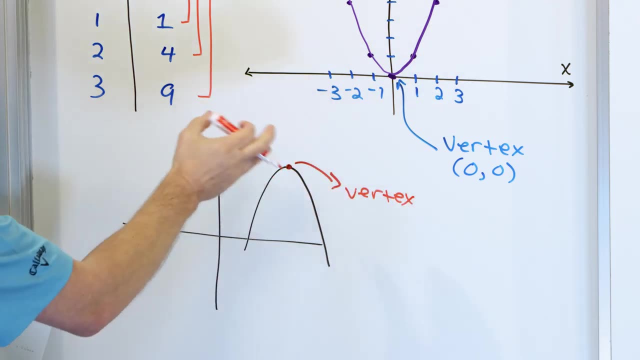 In this case the vertex would be whatever the maximum value was here We're going to call that the vertex So I can give it some coordinate points or whatever. I'll do some more detailed example later. But this coordinate might be like five comma six or something there. So the vertex. 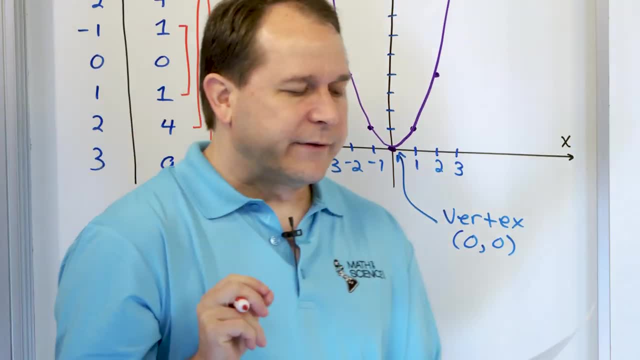 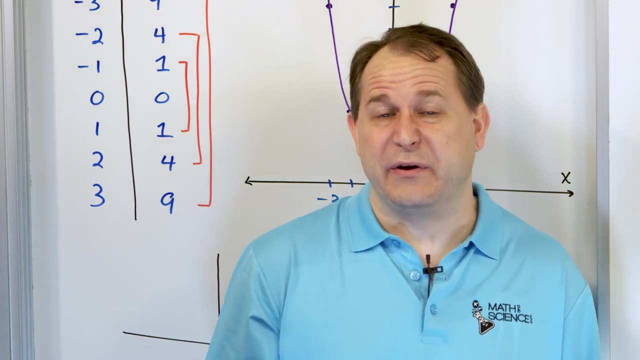 is basically the maximum value. Now, the other thing that I want to talk to you about is what we call the axis of symmetry. It has a very complicated sounding name, but it's actually very, very simple. Okay, this thing- another way to say it, instead of calling it an axis of symmetry- is you can think of 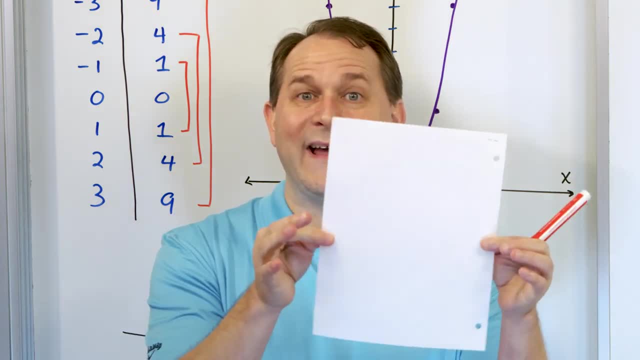 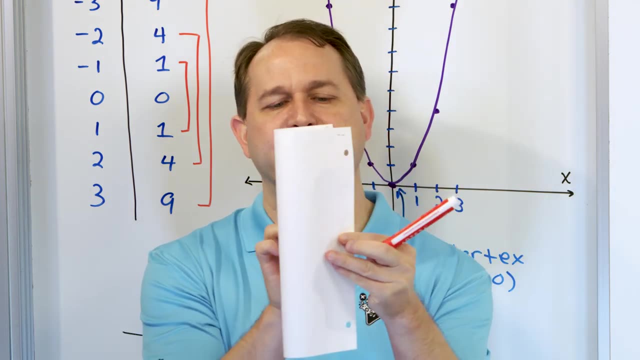 it as its mirror image. right, This piece of paper is erected, It's a rectangle. right, This piece of paper is symmetric, It has a symmetry to it. right, Because why I can take this piece of paper and I can fold it in half, And so this piece. 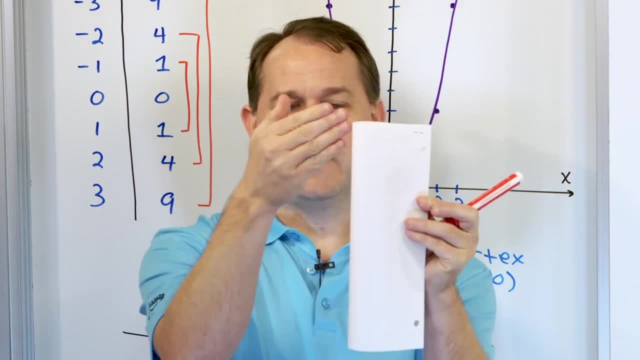 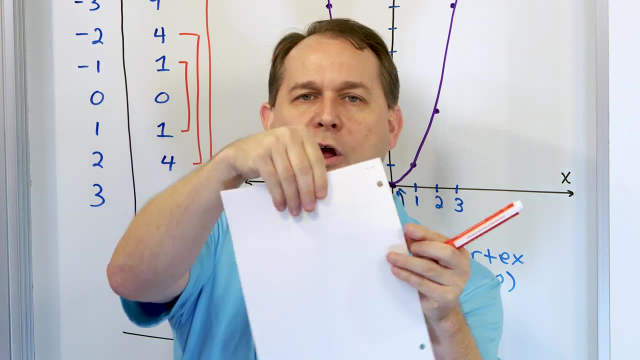 of paper has an axis of symmetry along the long direction. You know, if I could draw a dotted line, like through this piece of paper, I have an axis of symmetry of this thing because I can fold it into mirror image. Also, if I turn the piece of paper sideways, I have 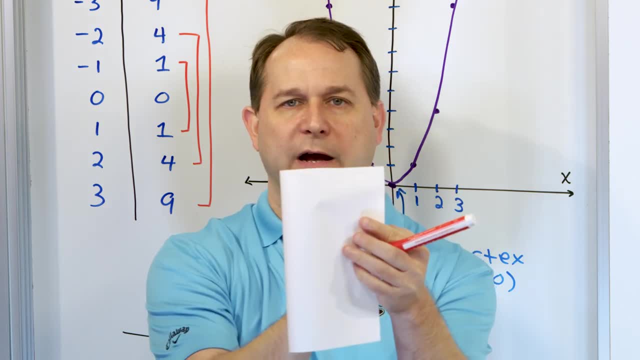 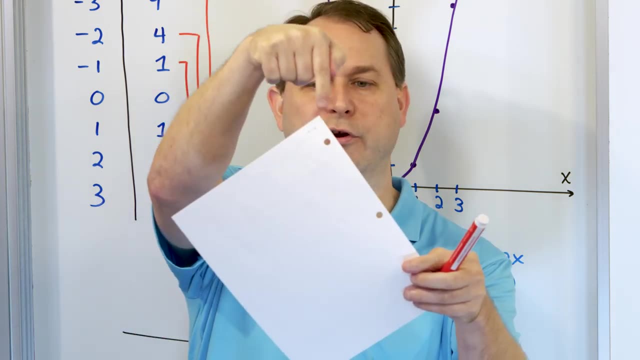 an axis of symmetry going like this, because I can fold it across. Now, of course, not every line is an axis of symmetry. For instance, let's say I have an axis of symmetry here. If I try to draw an axis of symmetry through the corners like that, it doesn't quite work. 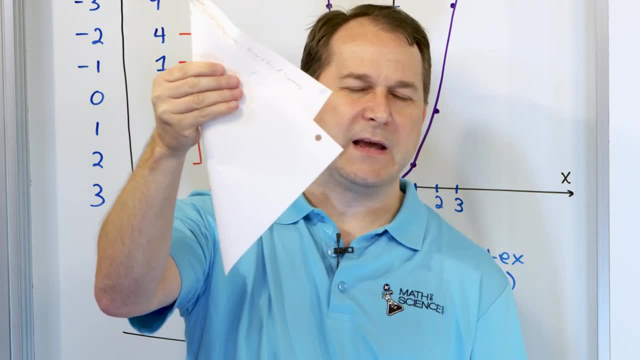 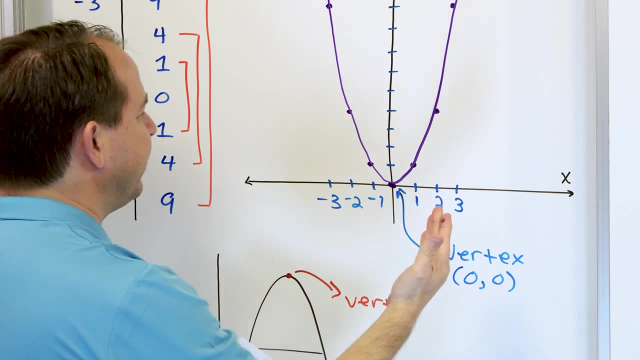 because if I try to fold it from corner to corner you see it doesn't really line up. And the thing has to line up exactly for it to be a mirror image or an axis of symmetry. So this parabola has a very special axis of symmetry. This one does as well, And you can. 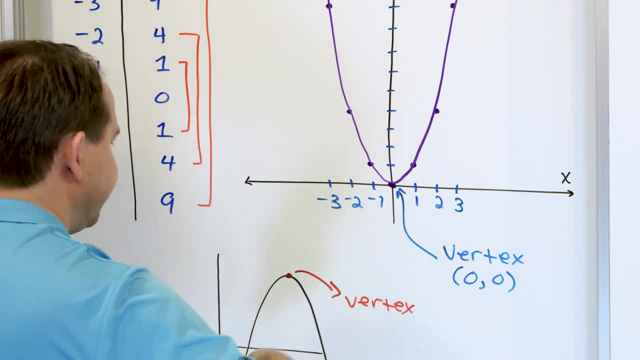 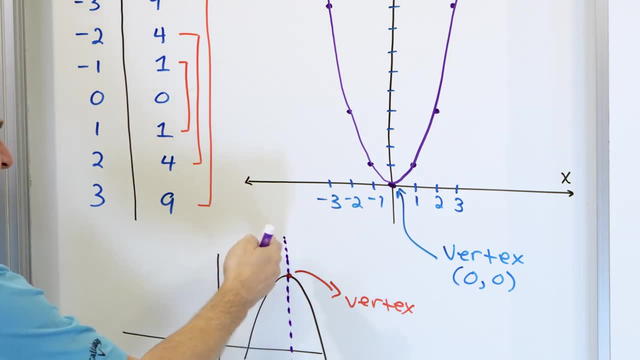 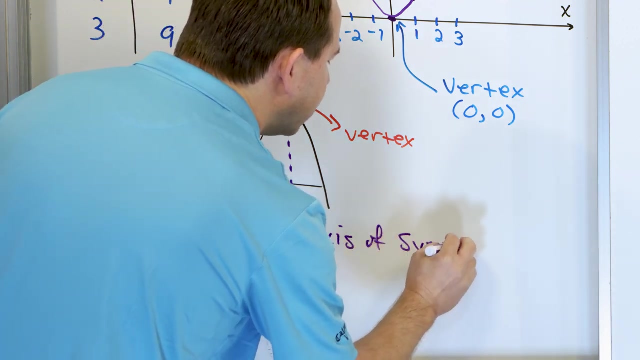 see that that axis of symmetry is a line like this that goes vertically and cuts, goes right through the vertex. It always has to go through the vertex, which is the center, And this is what we call the axis of symmetry. What it means is: it's the dotted line. that I can. 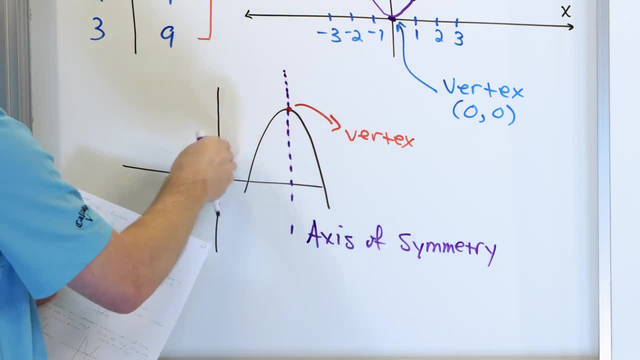 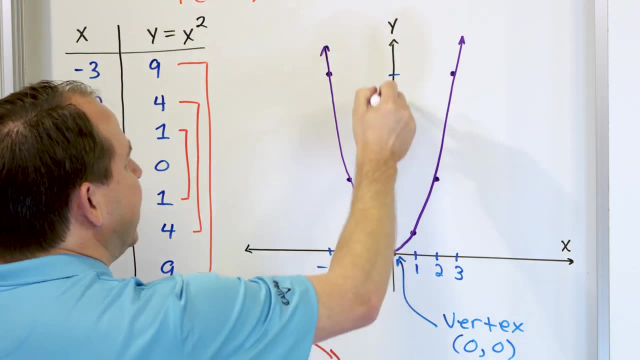 fold that parabola on itself and have it perfectly lined up. There's only one axis that works and it goes right through the vertex. The axis of symmetry of this parabola is the y-axis, right here, because the thing is centered there. I can fold this thing on itself Now before. 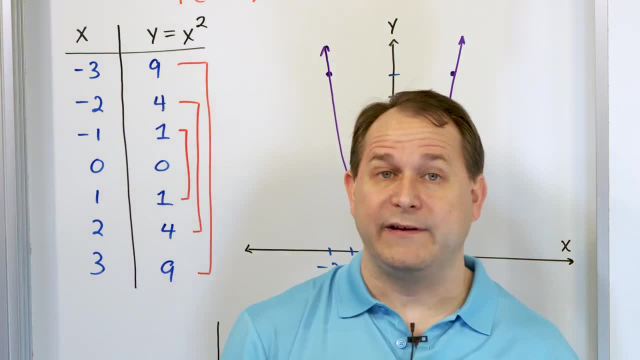 we close the lesson out. I've introduced the concept of what a vertex is. I've introduced the concept of what an axis of symmetry is. Now I just want to write down and sketch a couple of quick examples to show you numerically what these axes are, Because in your problems, your problem, might say: here's a parabola. 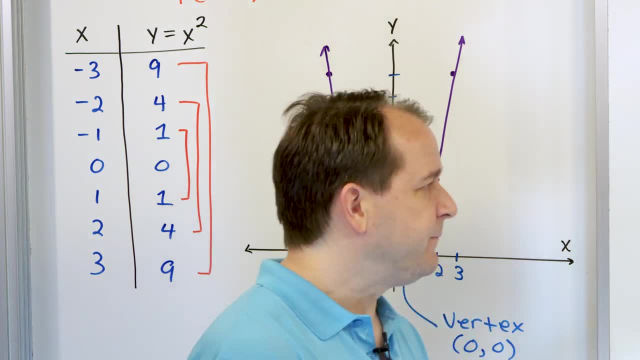 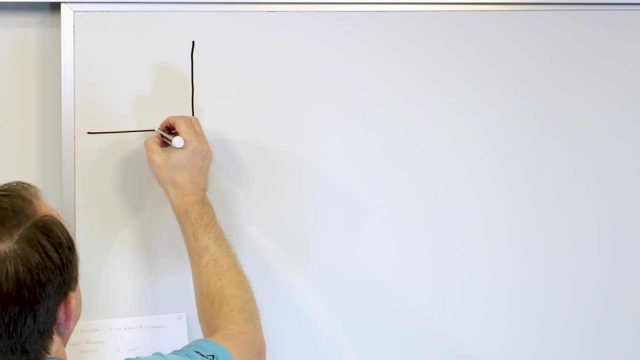 Tell me what the vertex is and what the axis of symmetry is, And you'll have to know how to do that. So let's go over here and do that. What if I had a parabola that looked like this? I'll go ahead and draw the axis, draw the parabola. We'll talk about what it is. Obviously, let's 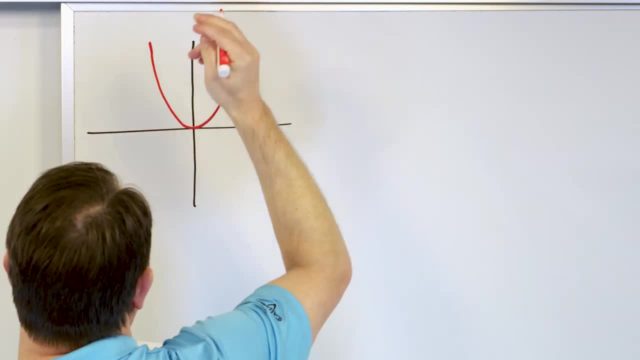 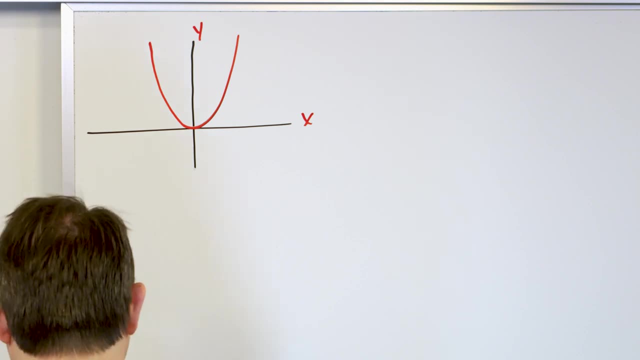 take a look at this parabola. It's going to be that nice, standard, beautiful parabola shape like this. Of course, this is x and this is y. This is kind of a gimme because we already drew it on the board here, But what is the vertex of this parabola? The vertex or the location? 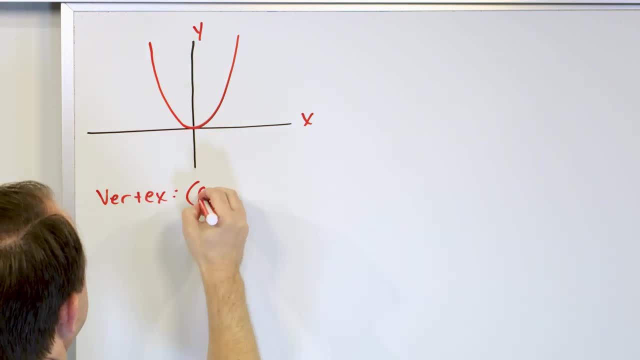 of the vertex is just the lowest point of the parabola And it's right here at the origin. So the vertex, just as we said before, is 0 comma 0.. The axis of symmetry. I'm going to write that as axis of symmetry. You have to express that as a line, because an axis 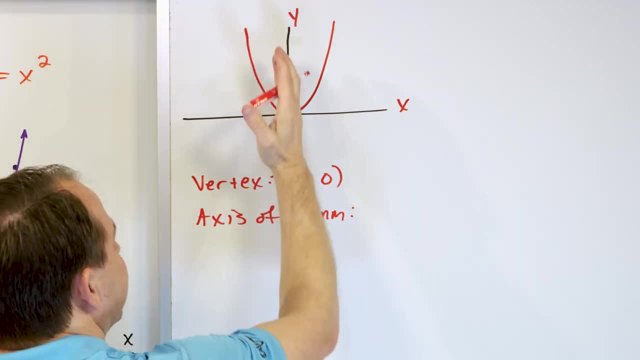 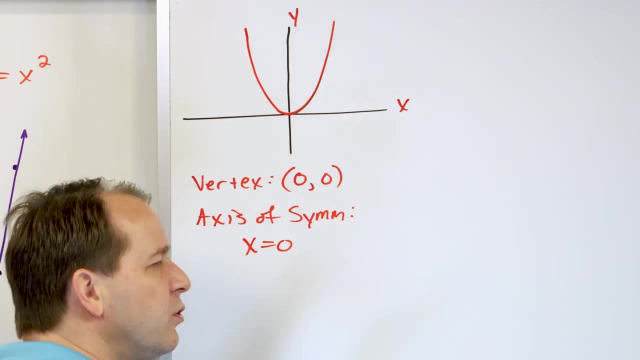 is a line right. But the line that is kind of the mirror image center point here is the line right here at x is equal to 0. Remember vertical lines in algebra. when you plot vertical lines they always have the same form: x equals something, right. If I have a line at x equals 5, that means 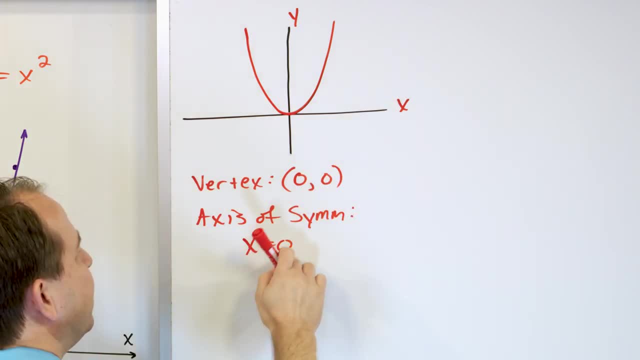 I have a vertical line over here at x is equal to 5, because the x values of every point on this line over here is at 5 units of x. right, In this case it's x is equal to 0 because the line is going right through x is equal. 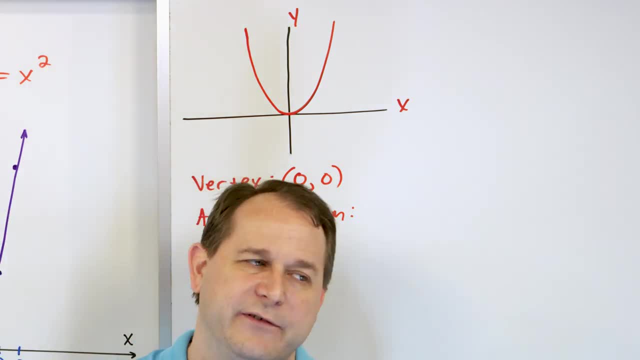 to 0.. I've talked about vertical lines in the past. You should know that, but I'm just refreshing your memory. So the vertex is a point, The axis of symmetry is a line, So this is not just an x value. 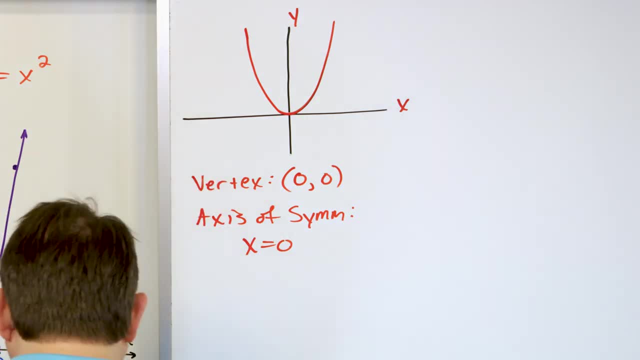 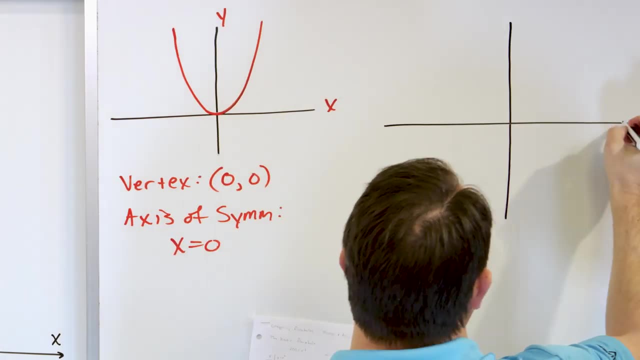 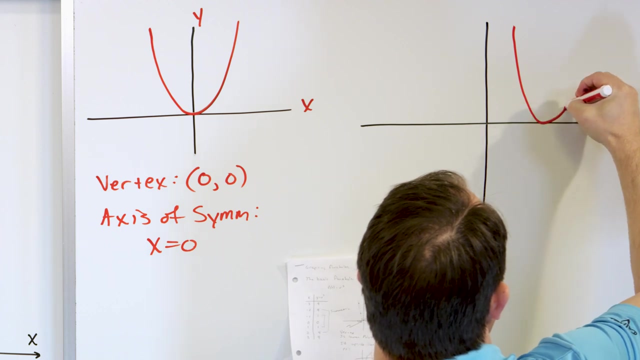 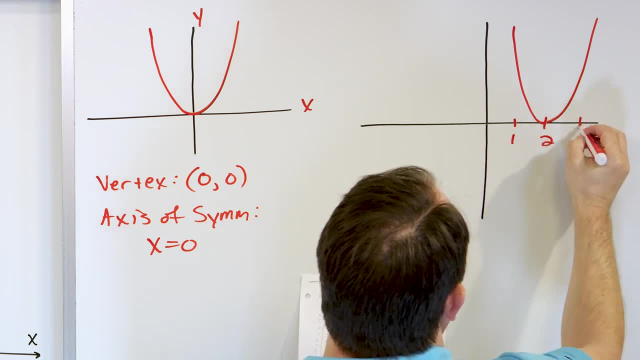 It's the same parabola. It's the same parabola, I'm just shifting it over. This is 1.. This is 2.. This is 3.. All right, So what would be the vertex and the axis of symmetry here? 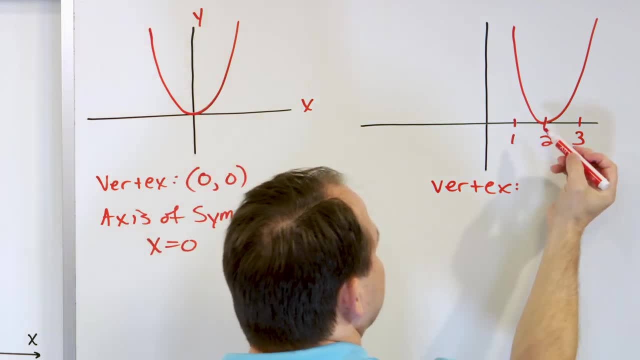 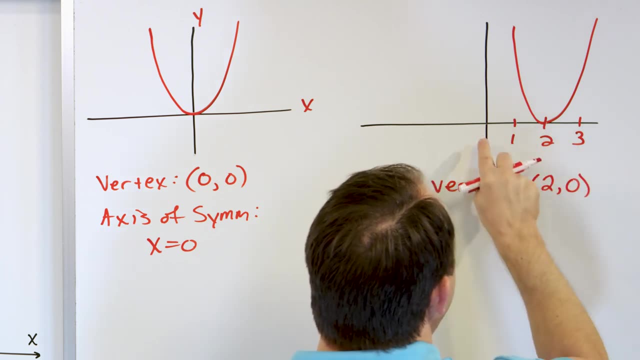 The vertex. what would be the vertex? Well, that's the lowest point, The point here. I've just shifted it from this point over here. The point over here is located at x is 2.. y is 0. So the vertex is now at a different location than the vertex before. 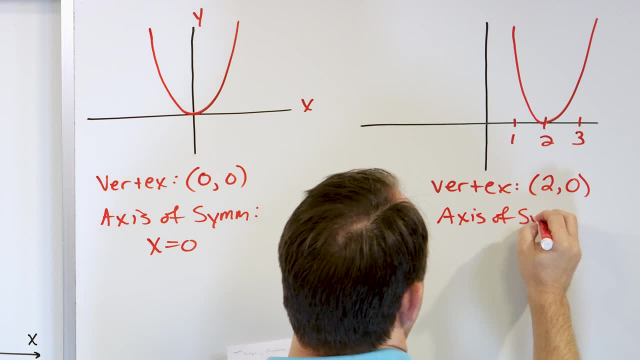 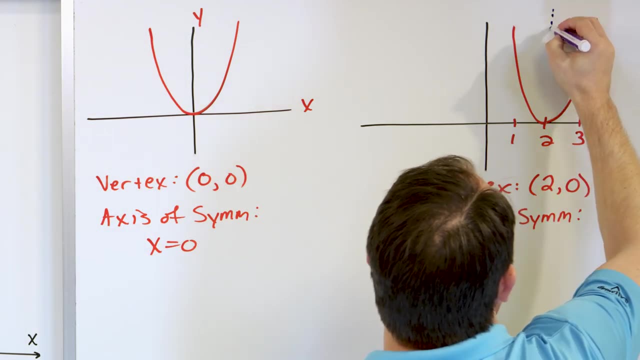 And the axis of symmetry is what? X Yeah, Yeah, It has to be a vertical line. right, It has to be a vertical line that bisects or cuts this parabola in half. It has to go right through the vertex. 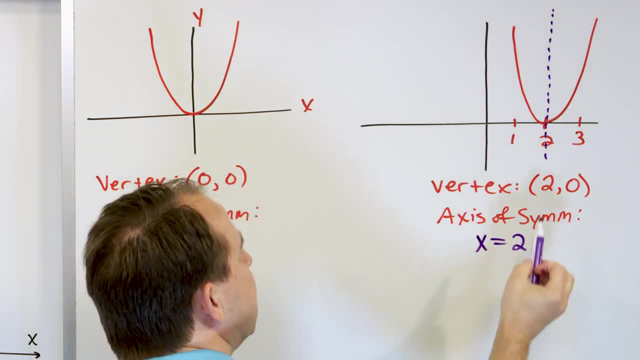 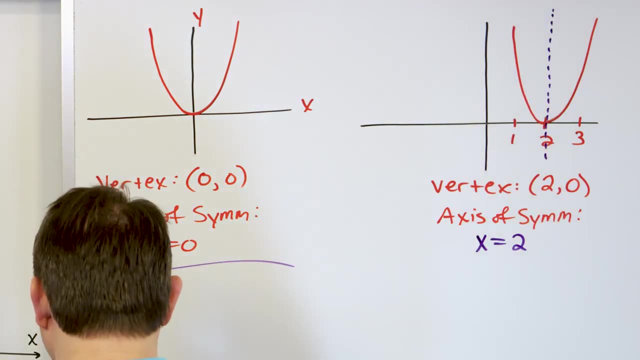 So the axis of symmetry is: x is equal to 2, because it's a vertical line located at x is equal to 2.. All the set of points that go through there, that's the axis of symmetry. So here we just basically took this basic parabola. 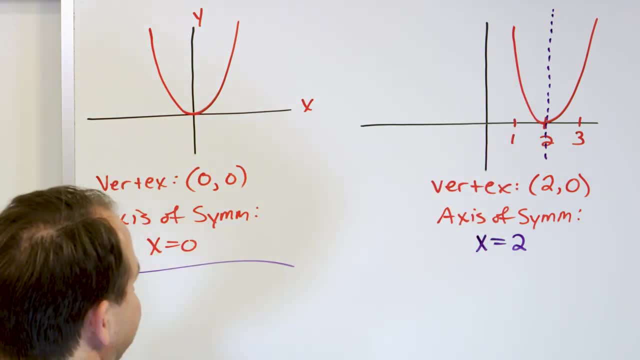 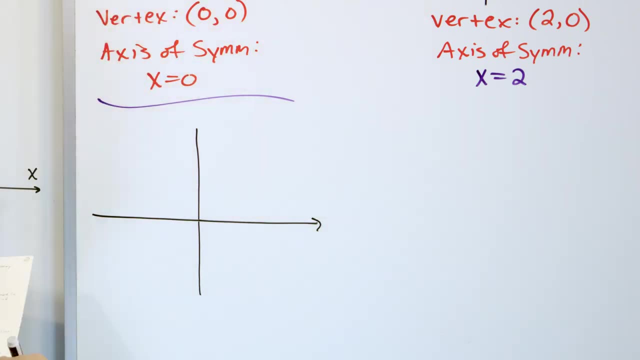 and we just shifted it to the right, And we can very easily see how to handle the vertex and so on. Now let's take and shift this parabola in a different location, entirely right. So instead of shifting it over here, let's draw the parabola. 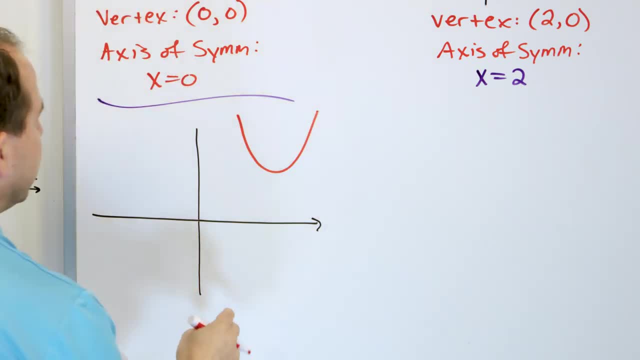 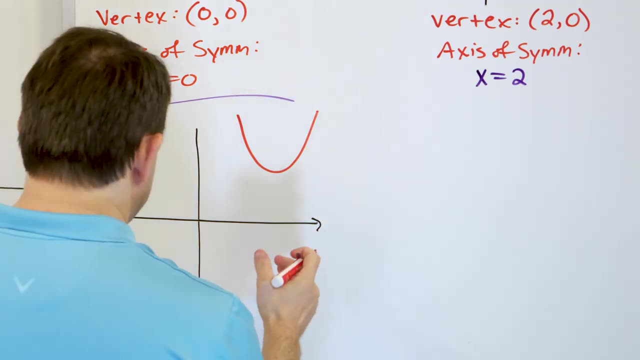 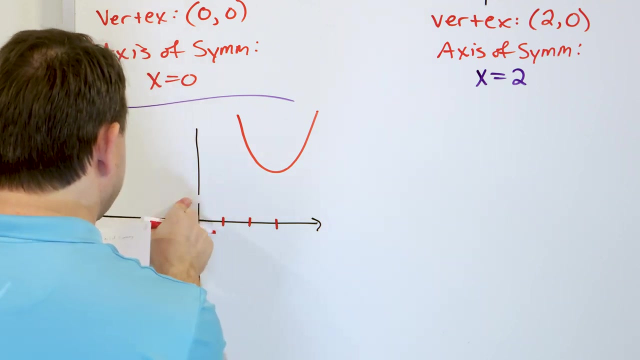 Let's draw the parabola way up here in space, something like this: So it's not on any of these axes. What would the vertex and the axis of symmetry be in that case? Well, you could say 1, 2,, 3, 1, eh, kind of mess it up. 1, 2.. 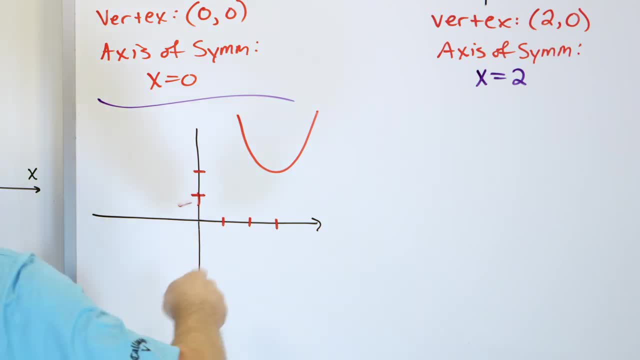 That's what I'm trying to go for here, like this. If I had drawn it, If I had drawn it like this, then I could kind of dot a line over here and dot a line over here, And this is at: x is equal to 3 and y is equal to 2, right. 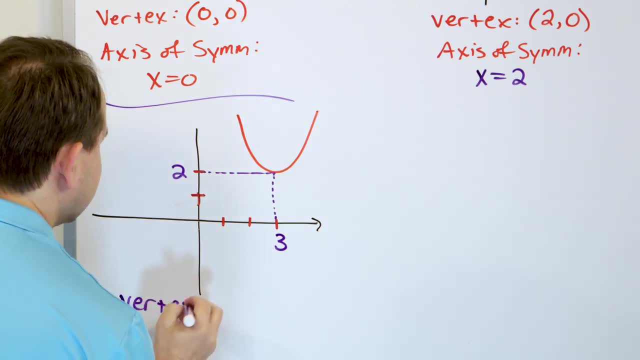 Then what would the vertex be? The vertex is just the location of this minimum point 3, 2.. Basically, you just read off the coordinates of where the lowest point of that parabola is. And then what would the axis of symmetry be? 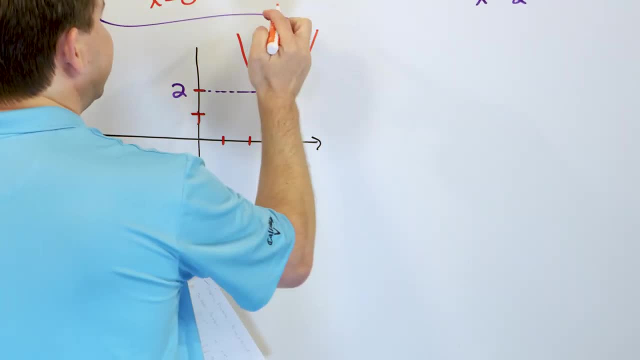 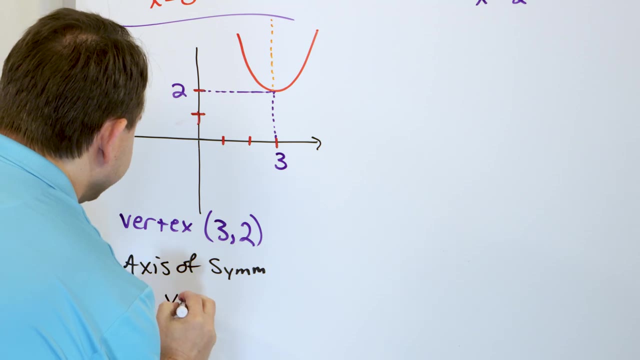 It has to be the vertical dotted line that cuts this thing in half and it goes right down. You can see it goes right through 3, right, So this axis of symmetry is: x is equal to 3.. So you can kind of see the pattern here. 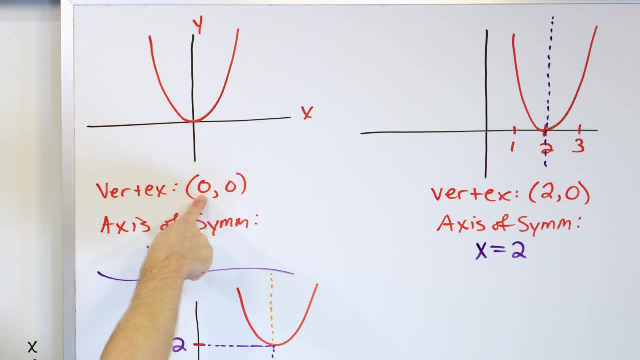 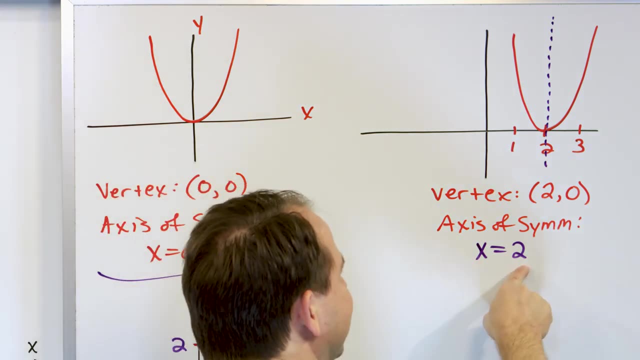 The axis of symmetry always goes through the first part of the vertex, because that's the x-coordinate of where the vertex is. x equals 0 goes through this point. x is equal to 2,. the line x is equal to 2 goes through the point 2.. 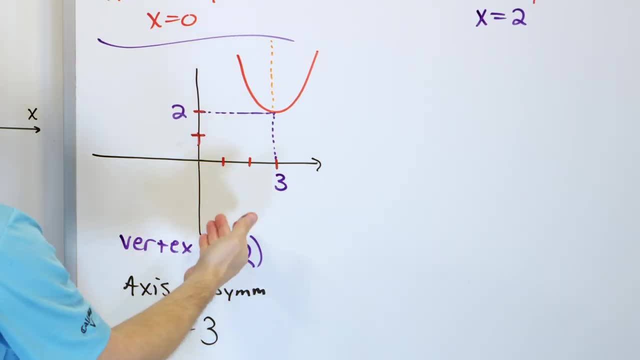 The vertical line, x is equal to 3, goes through this, So they all match. So the axis of symmetry is always going to be the first number in the coordinate, That's the coordinate of the vertex. Now, so far all of these parabolas. 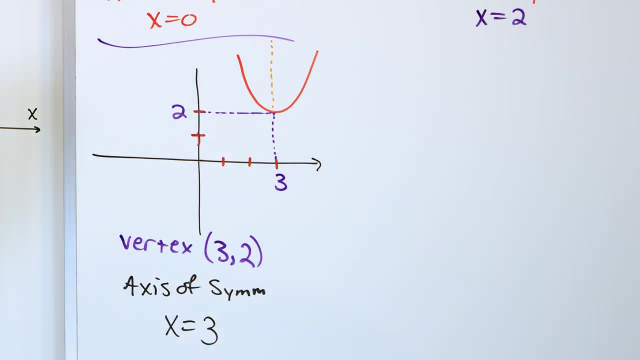 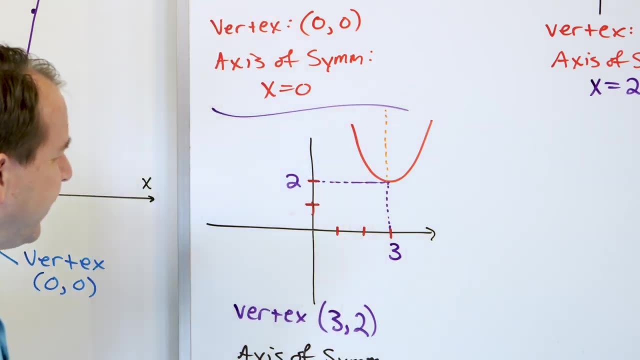 except for this one that I drew, have opened up, And we're going to find out an easy way to figure out if a parabola opens up or opens down later, But for now let's focus on what would? the vertex and the axis of symmetry. 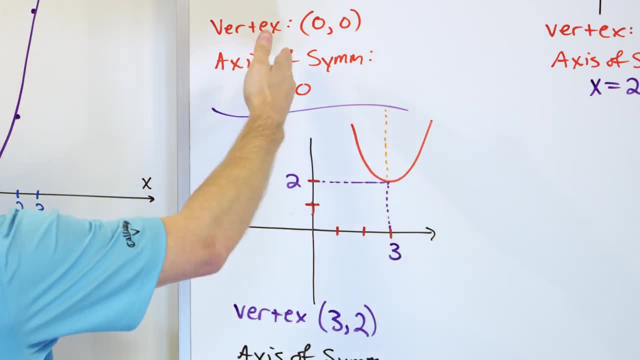 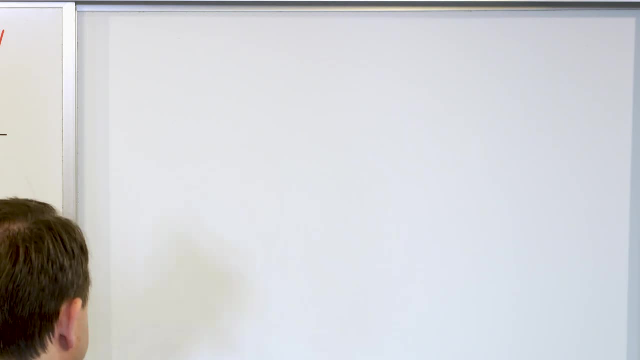 look like for a parabola that opens kind of upside down. So instead of a smiley face like all of these parabolas, what if it opens as a frowny face that goes upside down? So if the parabola goes upside down, 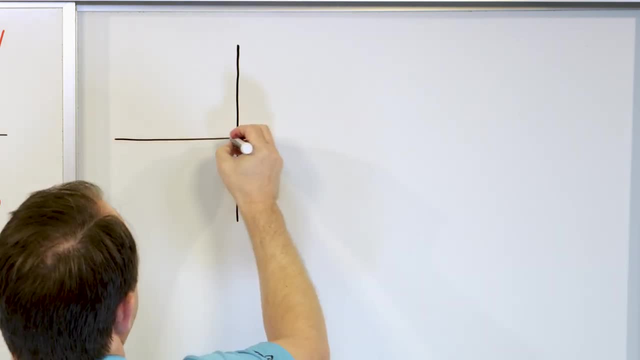 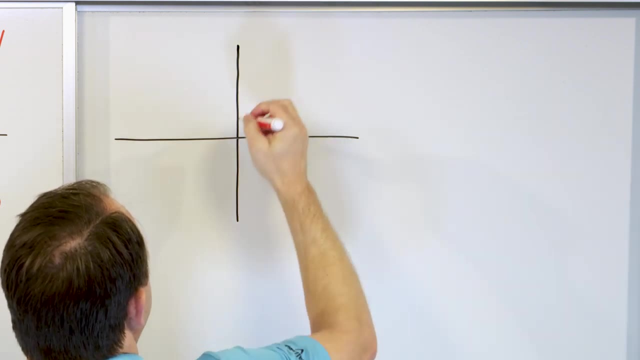 you might have something like this. So let's take a look at a quick sketch of one of these guys. And, by the way, it's not rocket science. It's not going to be any harder, right? So let's say the parabola instead of opening up. 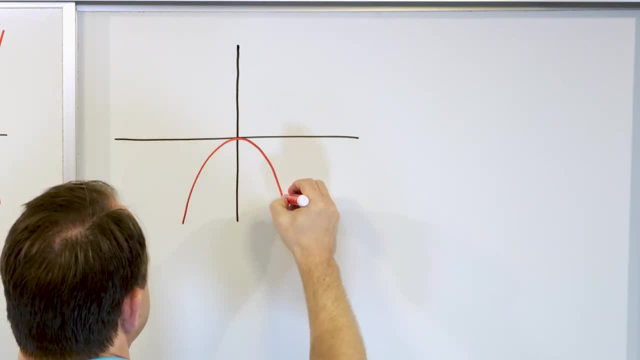 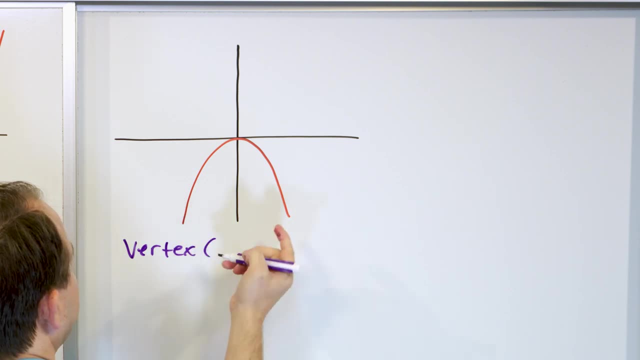 which is the standard parabola shape. it actually opens and comes down like this: What is the vertex and the axis of symmetry here? It's not a big surprise. The vertex is located at the highest point of this guy, which is right at the origin. 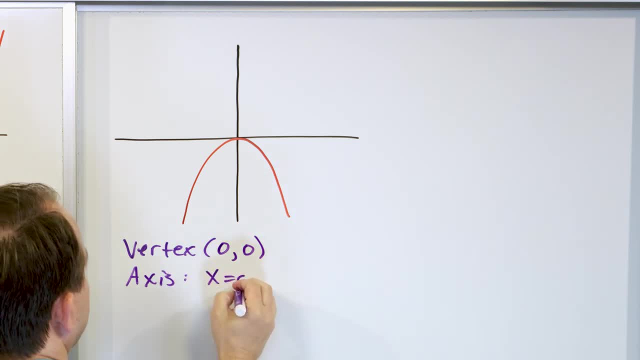 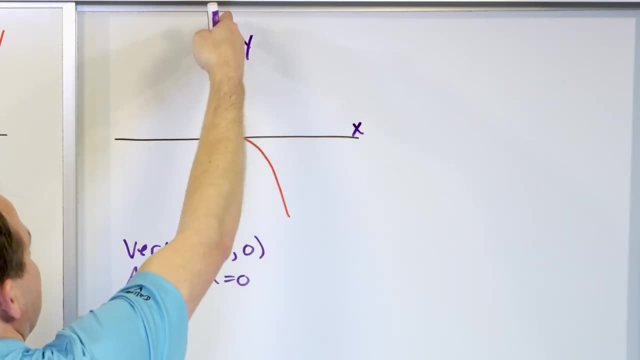 And the axis of symmetry is at: x is equal to 0, same thing. It's just the first coordinate here, because the line that bisects it is x is equal to 0.. Here, this is the x-axis, This is the y-axis. 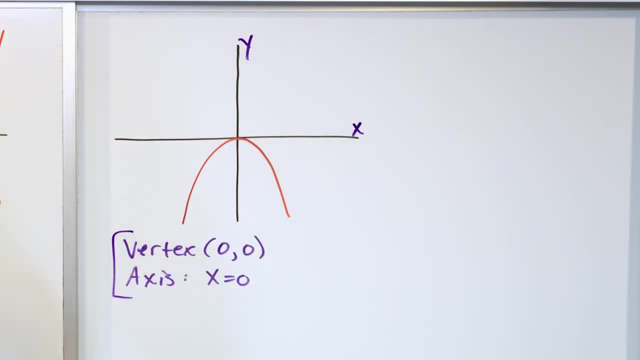 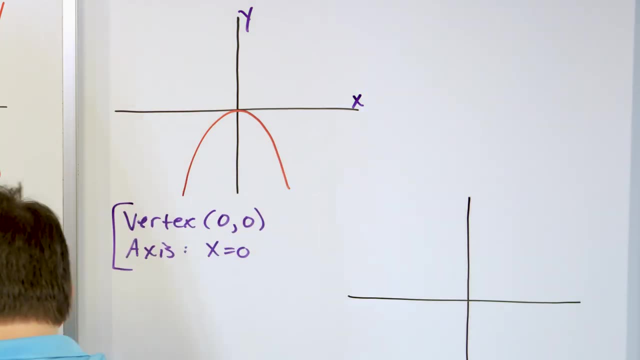 So x is equal to 0 here It goes right through there. That's the vertex and the axis of symmetry. And then we'll do one more before we close it down. What if we had a parabola over here? that let's try. 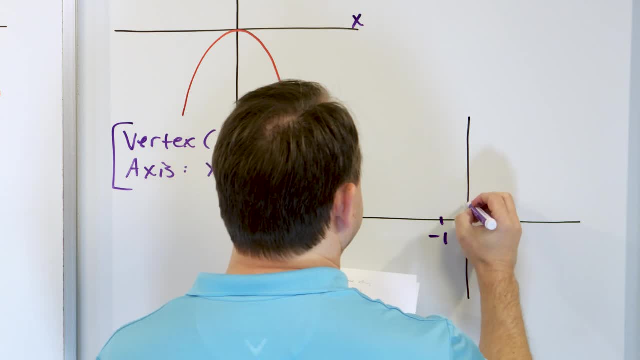 to be a little more precise, Let's say this is negative 1.. Let's say this is 1,, 2,, 3.. And let's say that our vertex is going to end up being there. So I kind of gave it away. 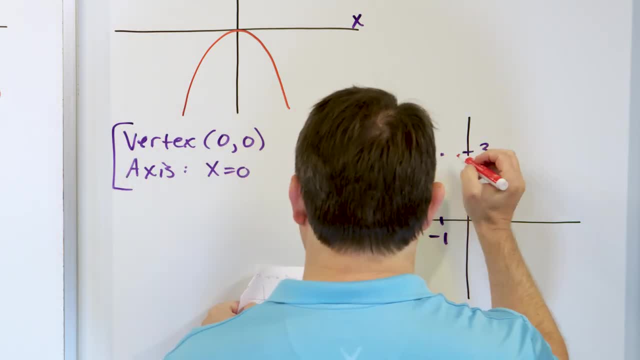 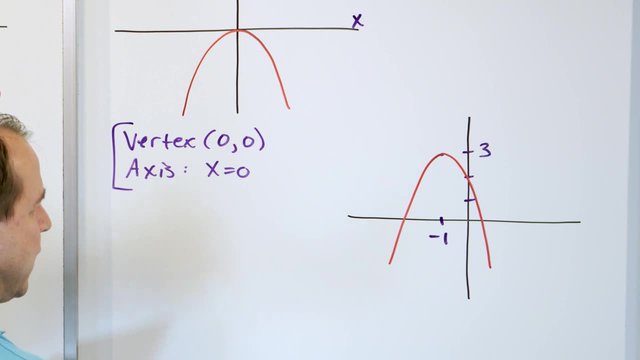 OK, Let's do that a little bit. But the point is that this parabola goes something like this, like this: It opens upside down: What's the vertex and the axis of symmetry? Well, you can see that the vertex is the inner. 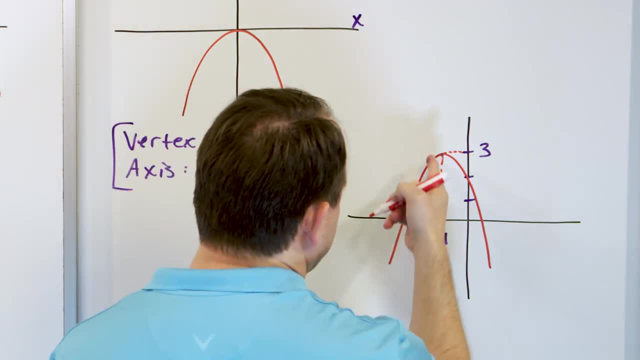 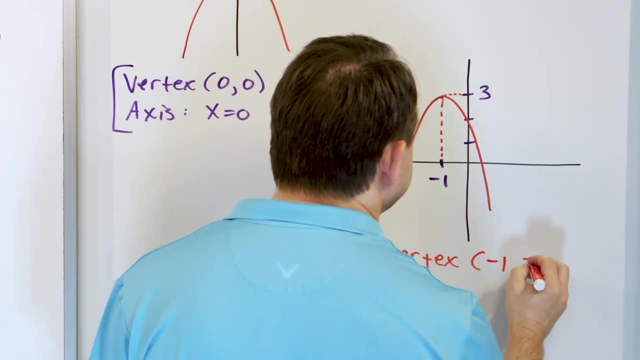 is the kind of where these kind of x and y values there the coordinates of this top point here. So the vertex is negative: 1, 3. That's x, y, And the axis is going to be this line. Whatever, this line is that. 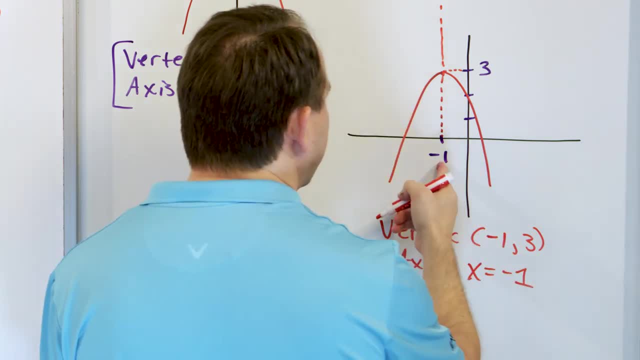 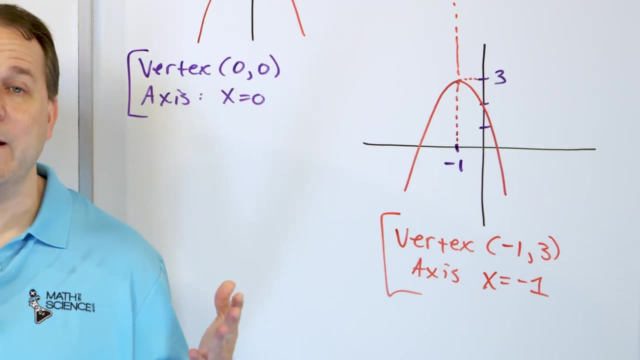 bisects. this thing, which has to be x, is equal to negative 1, right here, It's the one that goes through there. So this lesson was all about introducing concepts. We're going to be taking these parabolas that we've been learning about and we've